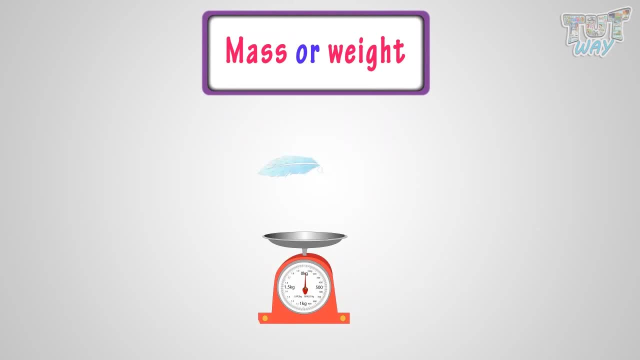 Here is a feather. it's weight is about just one gram. We write it like this: Here is a disposable spoon. its weight is about 5 grams. We write it like this: Here is a packet of some edible things. We test each packet with our beakerÓ. 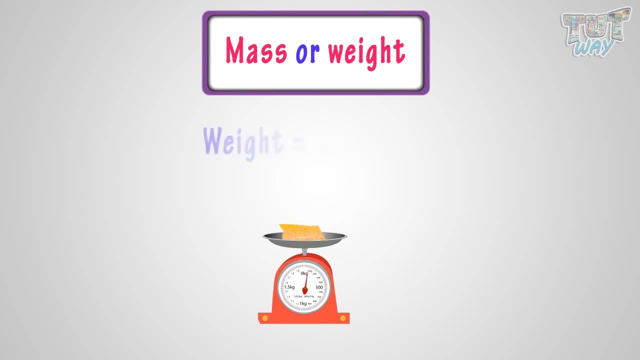 that weighs about 25 grams. Here is a small gift weighing 50 grams. Here are examples of some things weighing 100 grams. Here is a cake weighing about 500 grams- 500g. Here is an object weighing 1 kilograms or 1 kg, So we calculate the. 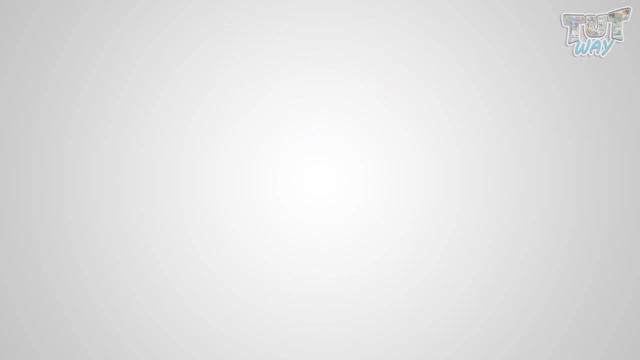 mass of objects by measuring its weight. Now let's try to remember a few things: 1 kilogram is 1,000 grams, 500 grams is 1.5 kg. 500 grams plus 500 grams will be 1,000 grams or 1 kilogram. 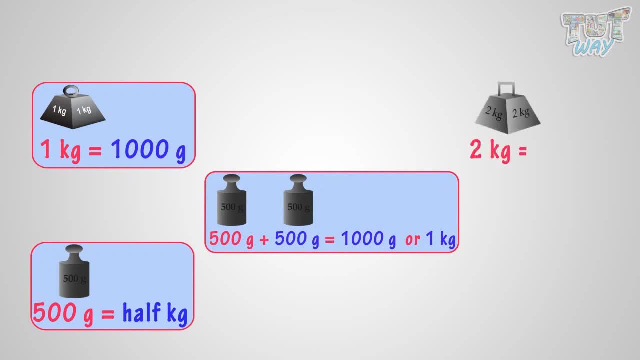 2 kilogram is 2,000 grams. 3 kilograms is 3,000 grams. 1 kilogram is 1,000 grams. 2 kilograms is 2,000 grams. 2 kilograms is 2,000 grams. 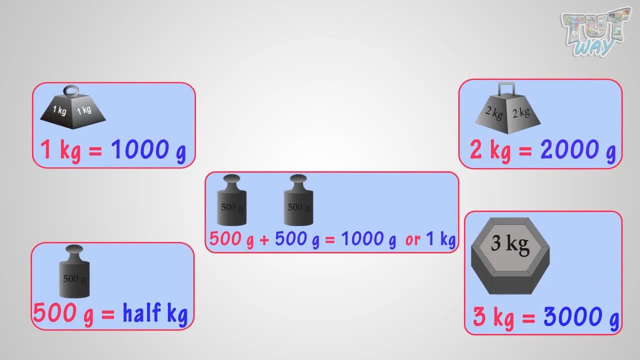 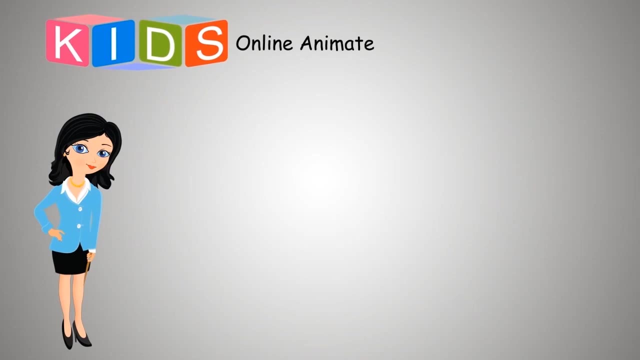 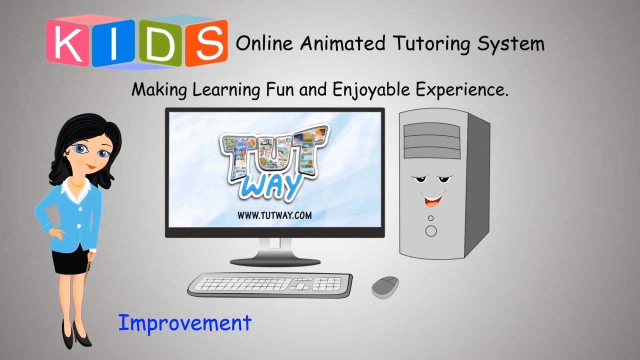 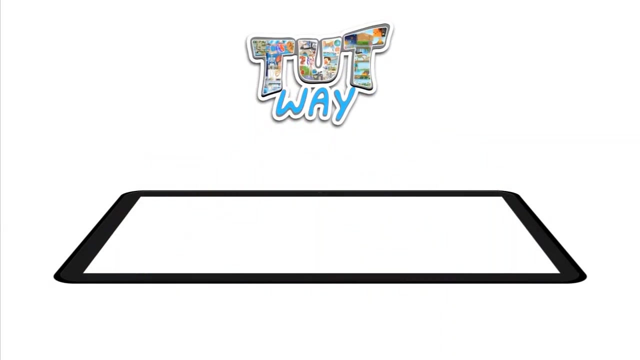 grams. Good So, kids. today we learned what is mass and how to measure it. Now go ahead and take a quiz to learn more. Bye, bye.